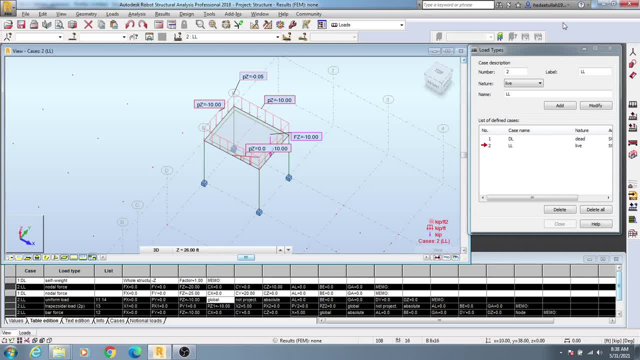 Dear civil engineers, in this lecture I'm just going to show that if you need to delete any types of load, Okay, if you need to delete any types of load from- I mean you have already Defined and how will do that. actually, it's very, very easy in robot to delete a load. 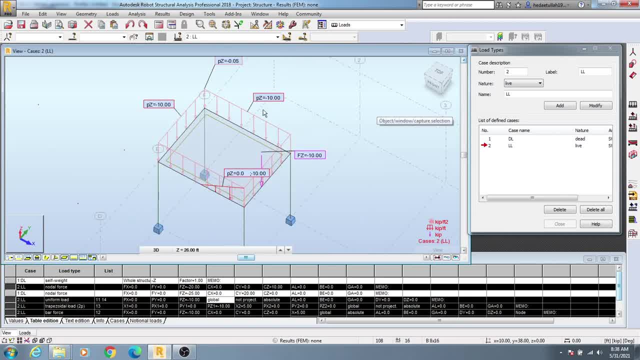 Just simply which load you want to delete. suppose I want to delete That one. Okay, so that's panel load. then simply come here. Then see: select from here. Okay, after clicking here, select our right click And Click delete. This is on option, Just simply see. 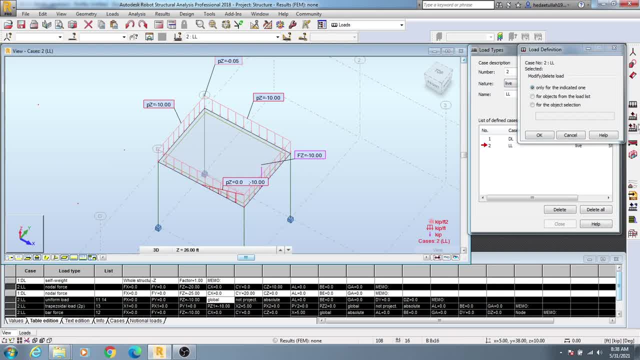 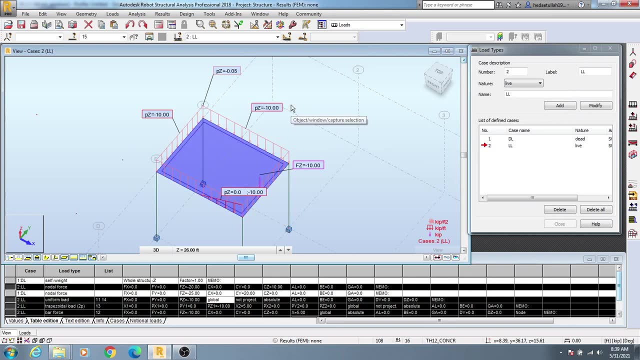 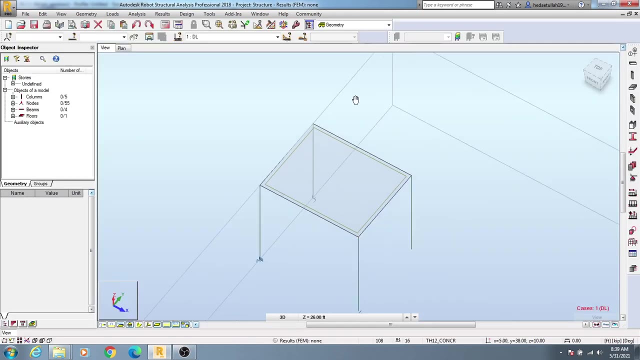 we have deleted that load, but After that just only for the indicated one. then Okay, just see our that load Have been deleted, So I'll just press ctrl Z To back. and again they have another option. just go ahead, geometry, Okay, and click here that option, that for. 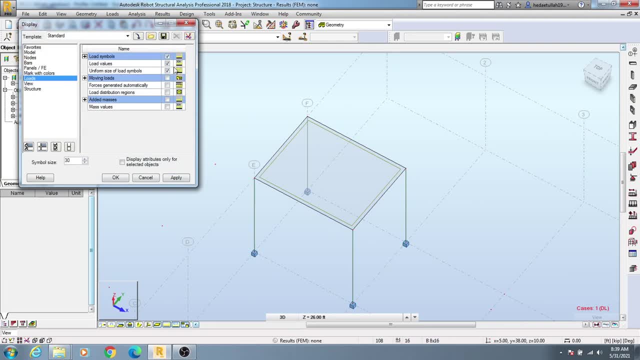 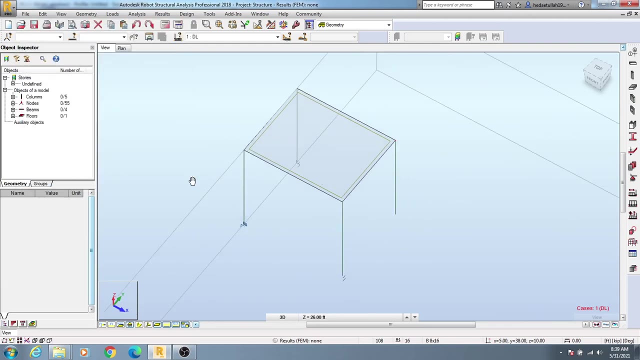 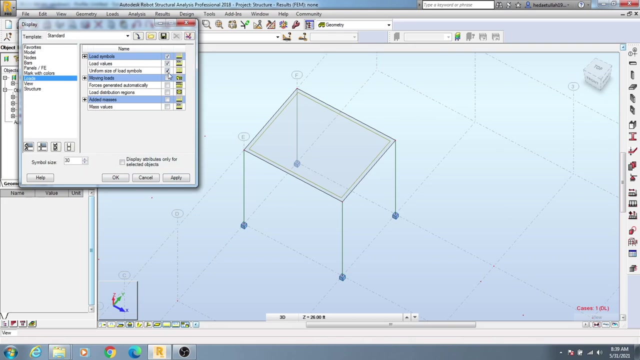 Size bar and click here load and from here click That option. Okay, so from here. from here, Simply click apply and click ok And again just go ahead. view and Display. from here load. Okay, just load sample. select all of that option, Okay, and 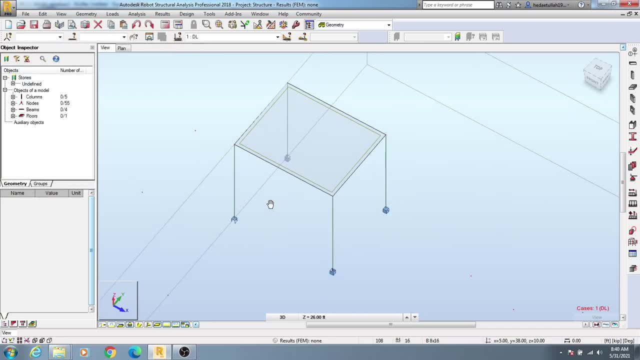 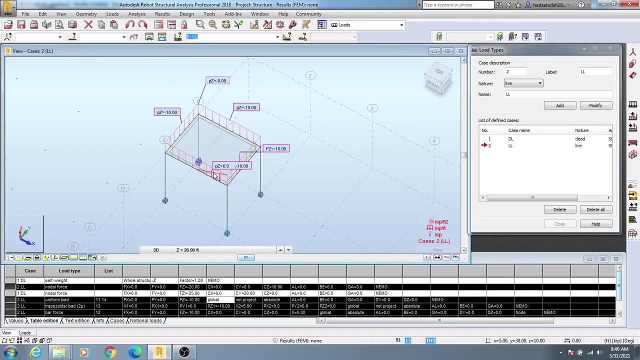 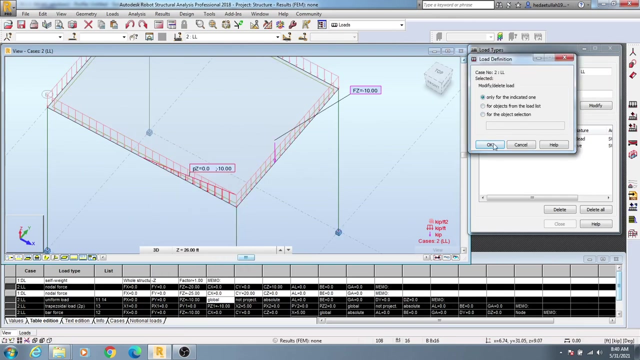 Apply. okay again. go geometry, Then load properties and from here select any of that load. suppose if you need to delete that Uniformly load from here after Selecting that load, like that, after selecting that load, right click and click delete, and just only for the indicated one, then okay, just see. 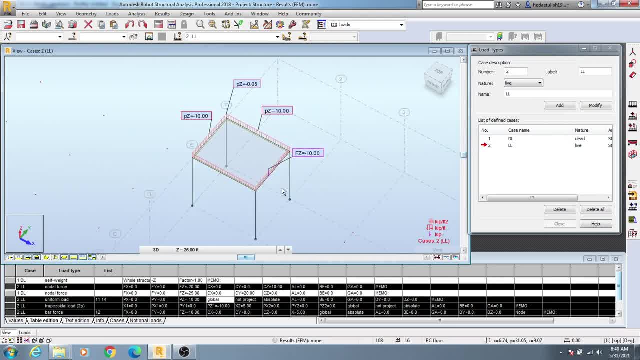 We have deleted on that particular load. So that is the way to delete, or this is the way to Do that particular text, that how will delete our required load. So thank you, Thank you very much. Still stay connected till next video You.